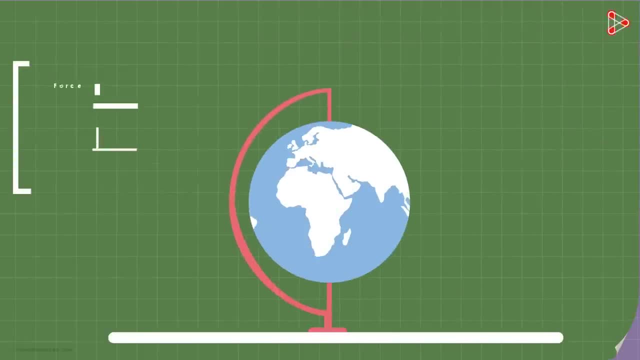 OK, Let's say there's an object on a table, You apply a net force of ten units on it, And then you apply a net force of twenty units on it. In which case do you think the acceleration will be more? Of course, the one in which the force was more. 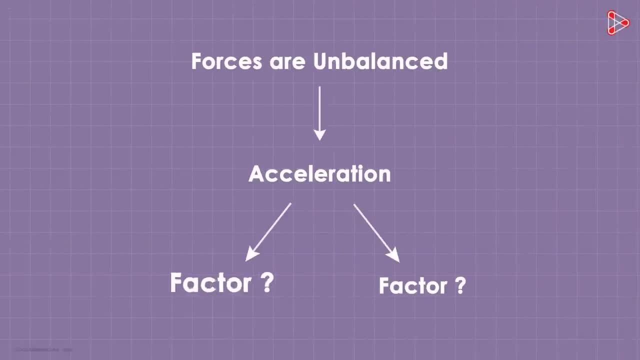 So we can say that one of the things the acceleration depends on is net force. If it's more, then more will be the acceleration. If it's less, then lesser will be the acceleration. OK, acceleration Acceleration depends directly on the net force. Come on now. I want you to 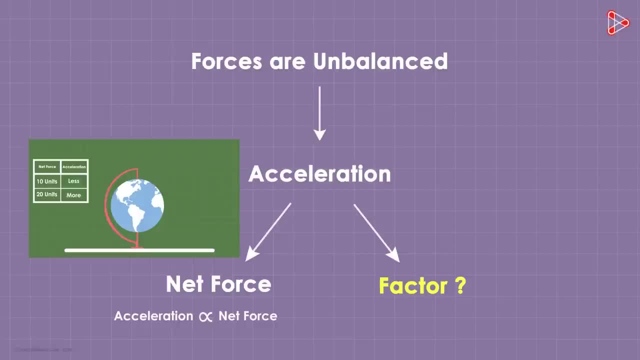 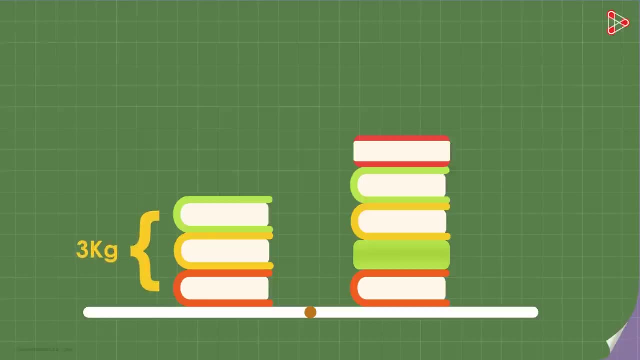 think about the second quantity the acceleration will depend on. Let's say there are two objects on the table. One has a mass of 3 kg and the other has a mass of 5 kg. Now, if you apply net force of 10 units to each of them, which one? 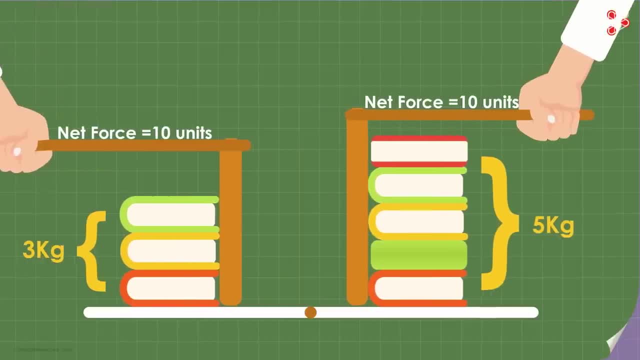 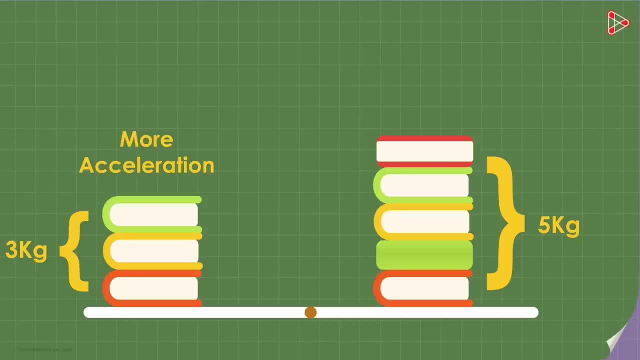 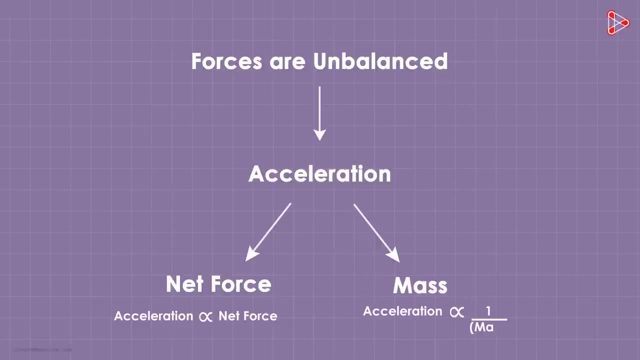 do you think will accelerate more? Surely it's the 3 kg one, because it has lesser mass. Lesser the mass, more the acceleration, And more the mass, lesser the acceleration. Hence we can say that acceleration depends inversely on the object's mass. 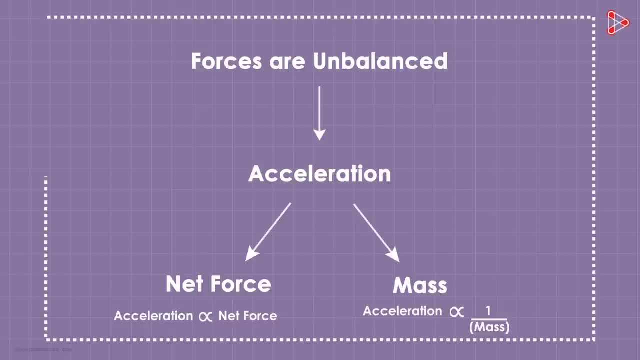 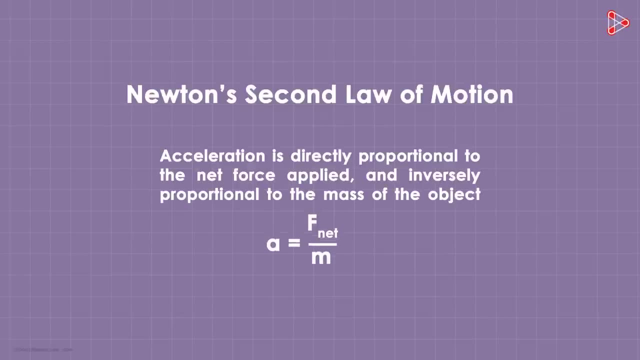 If you understand this concept well, then understanding the second law of motion will be very easy. Mathematically, it can be written like this In simple terms: the acceleration is directly proportional to the net force applied and inversely proportioned to the mass of the object. That's the second law. 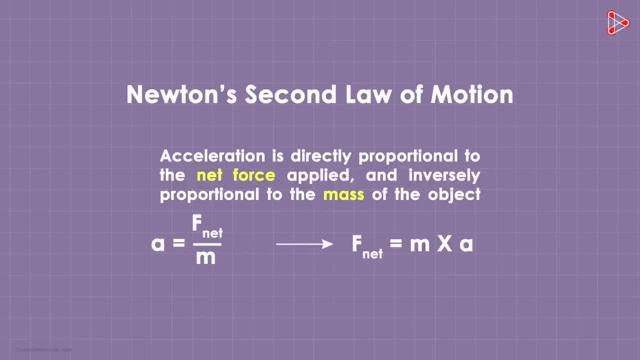 Or, as more people understand it like this: The net force is the product of mass and acceleration. With this, can you tell me the units of force? That should be easy. The standard unit of mass is kilograms And that of acceleration is meters. 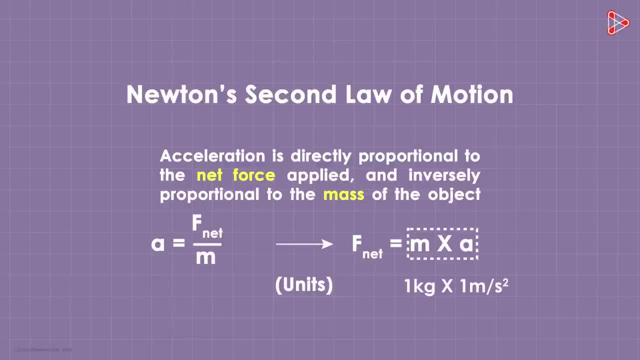 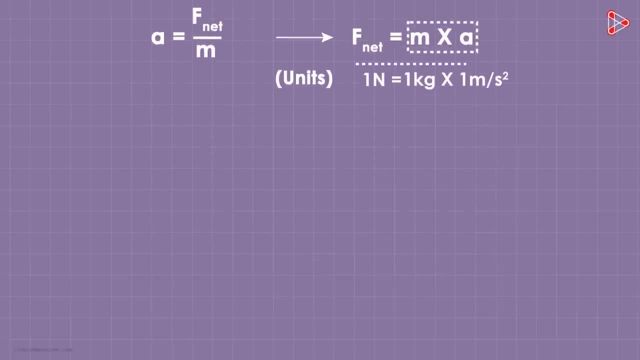 per second squared. So the unit of force is kilograms times meters per second, And this is what we call as Newton One. Newton is one kilogram times meters per second squared. So if the mass of the object is ten kilograms and the acceleration is ten meters per second, 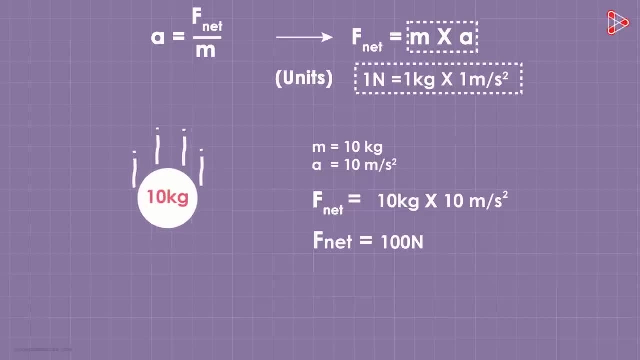 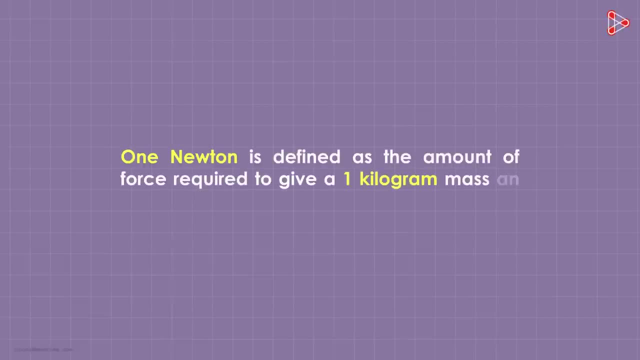 squared, then the force will equal one hundred Newtons. We can say that one Newton is defined as the amount of force required to give a one kilogram mass and acceleration of one meter per second squared. Subtitles by the Amaraorg community.